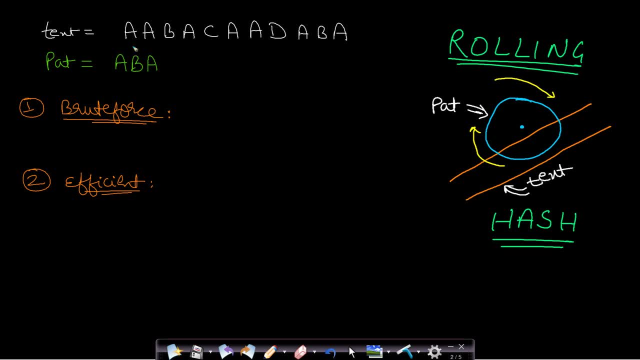 required to search for the pattern in the given text. In a very simple approach, what we can do is we can take a window size equals to the length of the pattern and then we can match each and every characters, and whenever there is a no match, then we will just break out of this loop and then 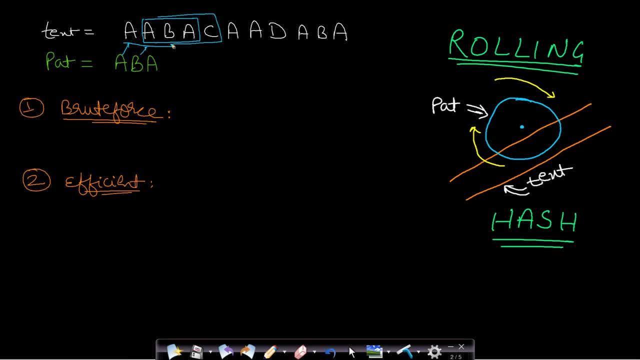 we will match the next window and then we will match the next window In the similar way we will do until we find a match. otherwise, if the text ends. So this approach will take order of length of the text, which is n, multiplied by length of pattern, which is m. So this will work in order. 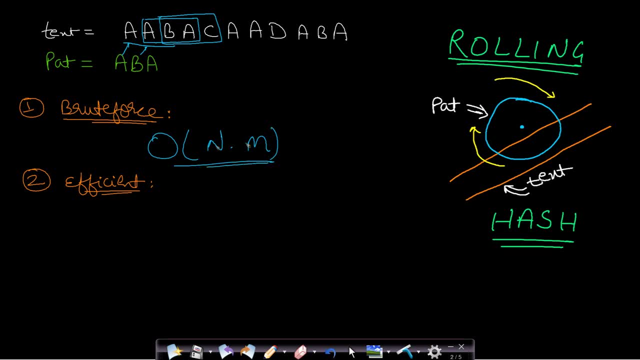 of nm time in worst case. Now what will be the efficient approach? The efficient approach will be by using the number of characters in the given text. So we will take the number of characters in the given text and we will take the number of characters in the given text. We will take the. 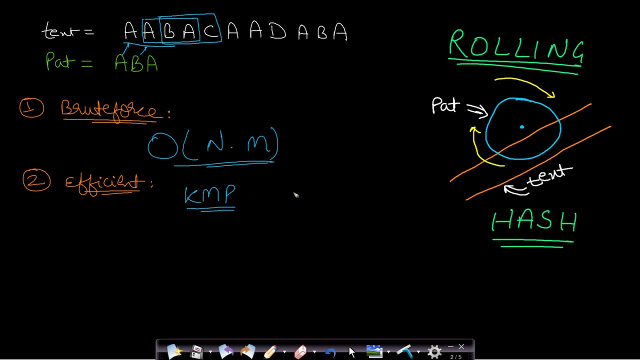 number of characters in the given text, and we will take the number of characters in the given text. Now what will be the efficient approach? The efficient approach will be by using the KMP algorithm, which I have already explained in one of my videos on sub list search and I will link it in the 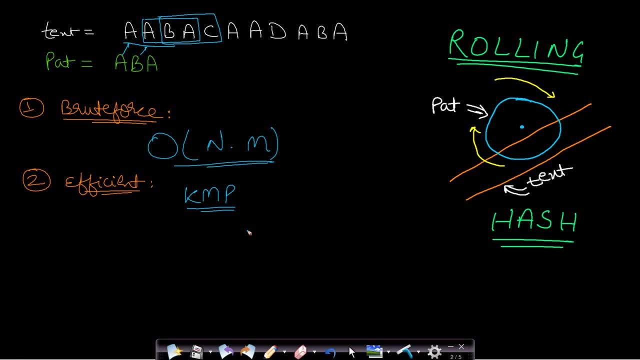 description below, so do check it out. An alternative approach to this problem is by using rolling hash technique. This technique is very similar to the case where we roll a ball on an inclined plane, So you will understand at the end of this video. So let us now look at the rolling hash technique. 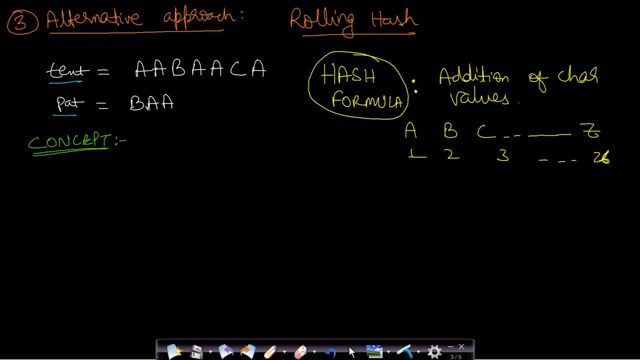 In this technique. let's say we are given a text as well as a pattern and we are required to find the pattern in the given text in the rolling hash. we will have an hash formula because we will be calculating a hash. let's say we are taking the simplest possible hash formula, which is just. 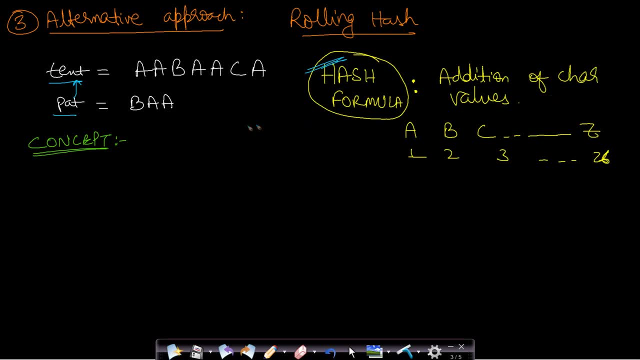 adding the character values in the window. so what will be the window size here? the window size will be equals to length of pattern, and in this case length of pattern is equals to 3, because it is having just 3 characters. so what we will do is we will calculate the hash value for pattern. it will 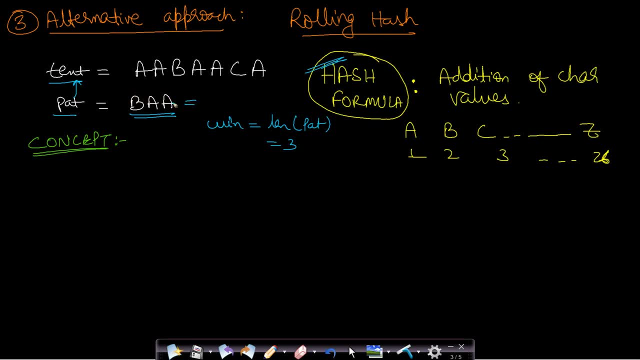 be nothing but the addition of values of these characters. and let's say we are taking the character values as a equals 1, b equals 2 and so on, to z equals 26, and how can you calculate it? let's say you are taking pattern at location i, then you will have to just subtract it with 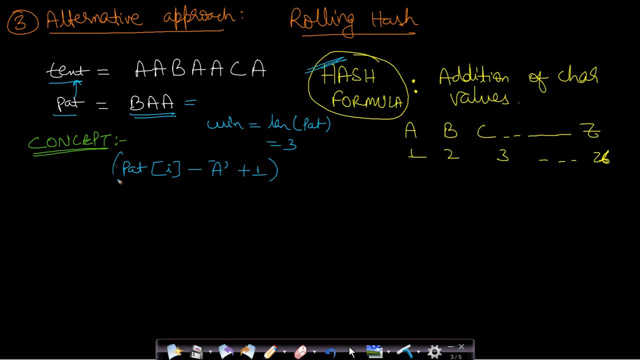 character a and then add one value to it and this will give you these values which we have assumed. okay, so in this way you can calculate the values. so what will be the value? for b? it will be two, for 8 will be 1 and for one another, 8 will be 1. so the hash value of the pattern of the place. 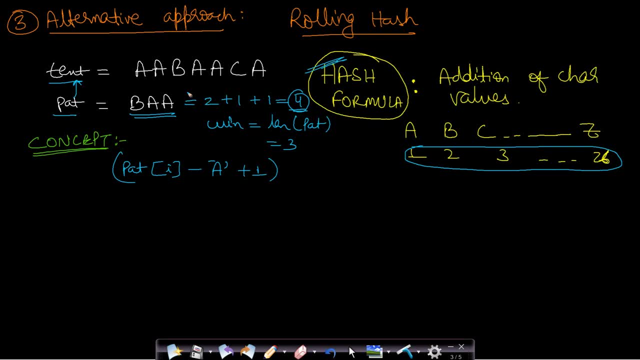 so the value of the value of the hash is always equal to the work case, which is 3, and it Erstñana pattern will come out to be 4. now we need to calculate the hash value of the first window. you can see that it will be 1 plus 1 plus 2, which will be equals to 4. now we will match the hash. 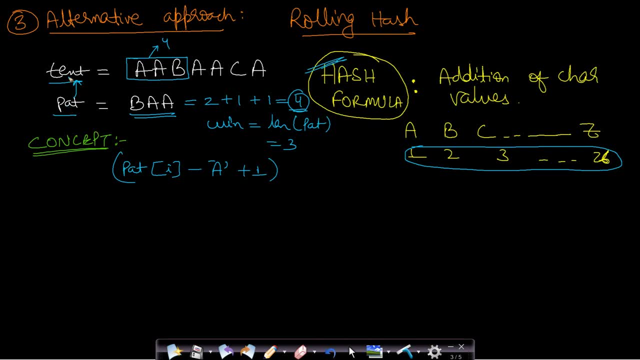 values of pattern as well as text. now, whenever there is a match of hash values, then we will match each and every character in this window and if all the character matches, then we have found the pattern. otherwise we will break out of this loop. so in this case, you can see that the hash value 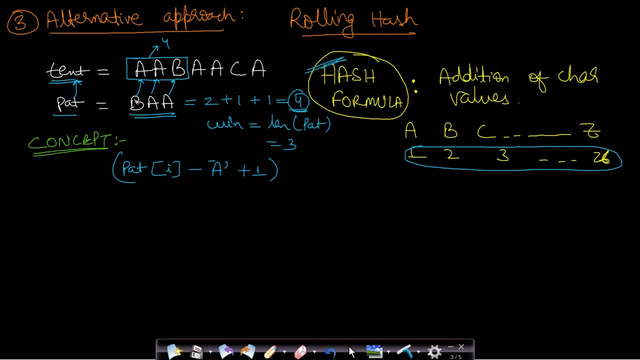 of pattern is exactly matching with the hash value of text, and so we will match each characters. since the first character itself is not matching, we will just break out now. when we break out, then we need to slide this window one character to the right. so our character now is a, a, b and we want 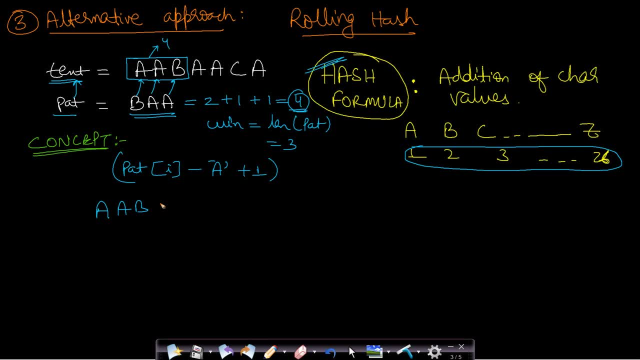 to slide it to the right hand side and include this new character, which is a. so when we want to include this new character, then we will have to leave out this left hand side character. now, how can we slide it, since we have taken the additive approach? so the value of a a b was 1 plus 1 plus 2, which was 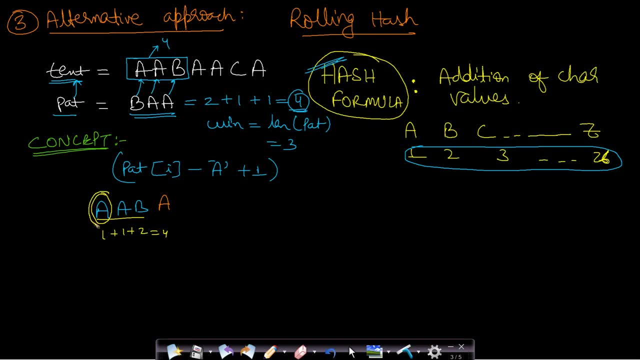 equals to 4. so we need to subtract the value of this leftmost bit, that is, a, and then we need to add the value of this a. so from 4 we will subtract 1 value will come out to be 3. now in this value, 3. 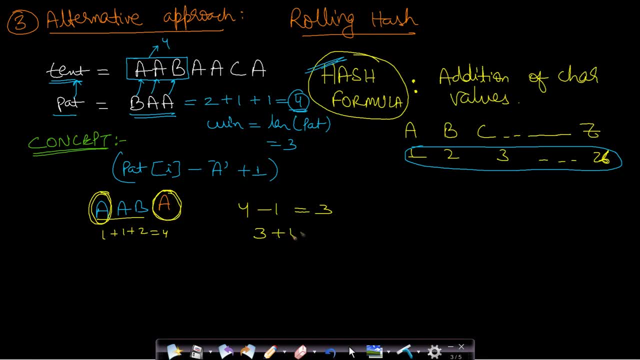 we will add the value of this a, which is 1, so again the value will come out to be 4. so the new for a, b, a will also come out to be 4. now again the pattern hash and text window hash values are matching. therefore we will have to match each and every letters character by character. so this will 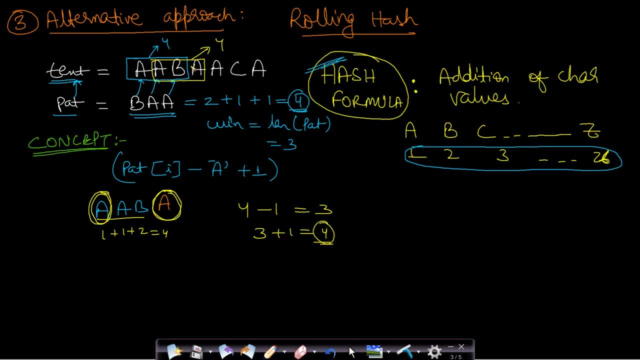 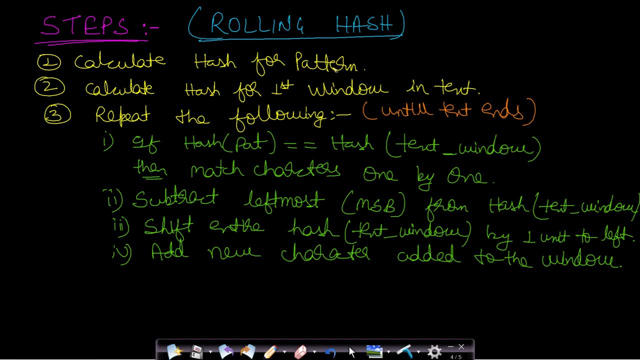 get repeated unless we find a match. otherwise the text window ends. okay. so i have written down the steps. you can see it here. first we need to calculate the hash for the pattern. once you have calculated it, calculate the hash for the first window in the text. once done, then repeat. 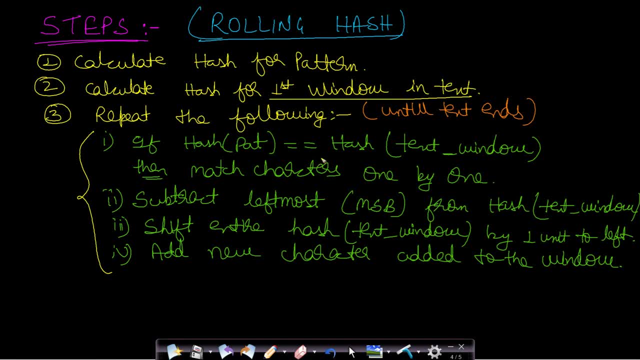 all these four steps, the hash pattern is equals to hash of the text window. then match characters one by one in the given window, and if there is a match then you have found the pattern. otherwise you repeat these steps as well. subtract the leftmost- that is the most significant bit from the hash- and then shift. 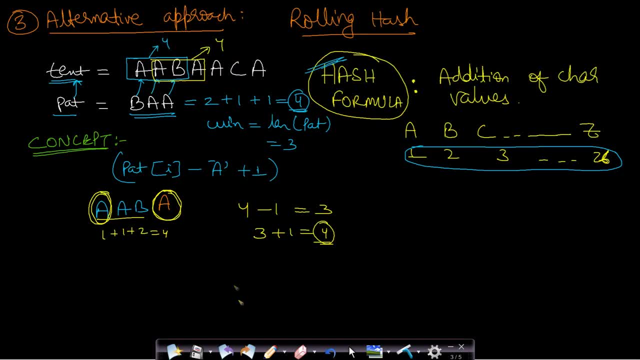 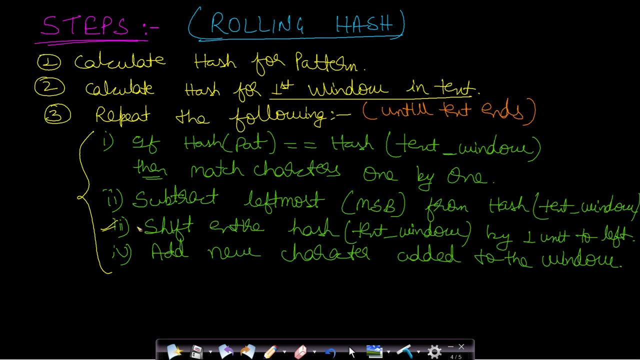 the entire hash by one unit to the left. so in this case we were shifting it to the left, but we had taken only additive values. so we don't require this third step for this technique. since this was a very trivial technique, i will show you the more advanced version as well. so in the 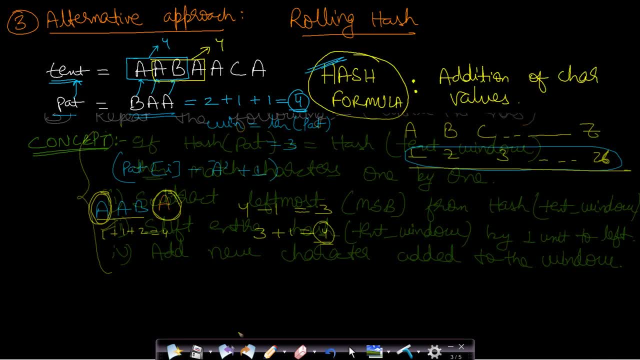 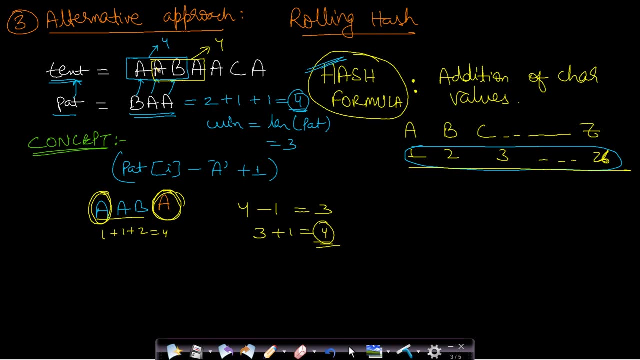 fourth step: add the new character added to the window. so we have added this a to the window value and again it came out to before now why it is called a rolling hash, actually for calculating the hash of the new window. we are not calculating the hash of all these characters, but we are just 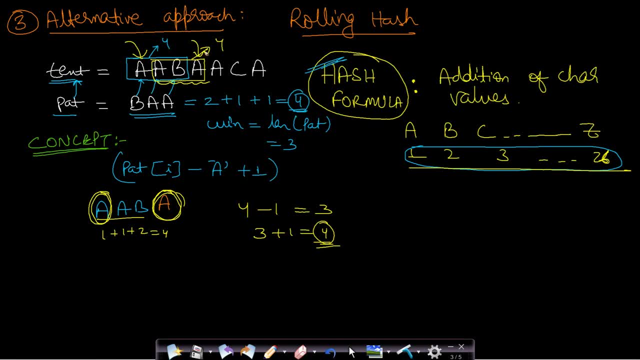 subtracting the last character and adding the first character. okay, so this is what we are doing. let's say your pattern length was equals to hundred. once you calculate the hash value for all hundred characters, then you can just slide it one by one, and you just need to add one character on the right hand side and subtract one character on. 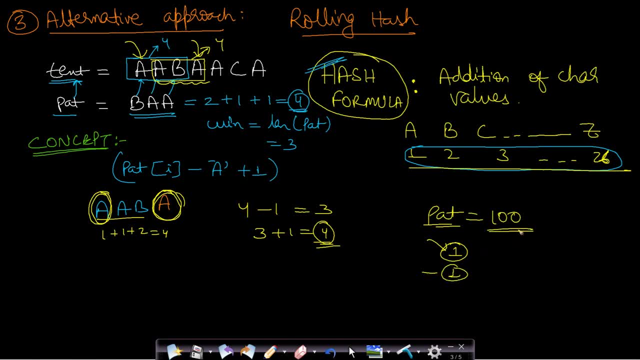 the left hand side. you don't need to calculate the hash value of the hundred characters again and again, so this will be a huge improvement. so this is what rolling hash is actually: when you roll a wheel to the right hand side, then if it acquires a pixel on the right hand side, then it 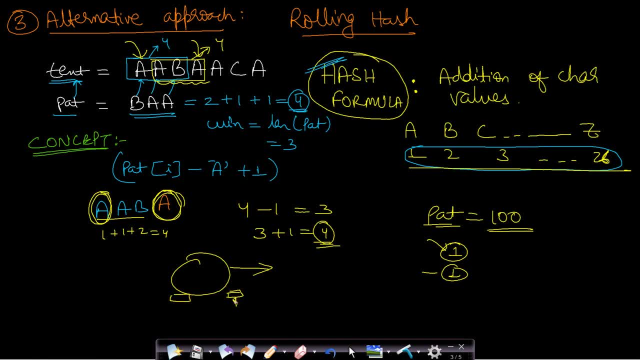 will have to leave the pixel on the left hand side. you can also call it a pixel on the left hand side, a brick or a block. so whenever it crosses a block, then it will have to leave the same amount of block on the left hand side, so this technique is known as a rolling hash. now there is a problem with this. 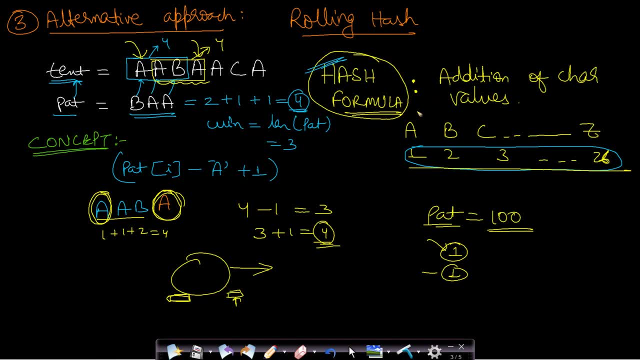 hash formula. actually, we have taken a very trivial formula and because of this we are getting a lot of matches. like you can see, that a a b is matching with b a a. even after jumbling this pattern, the additive values will all be the same. so this is a very naive hash formula and this will have a. 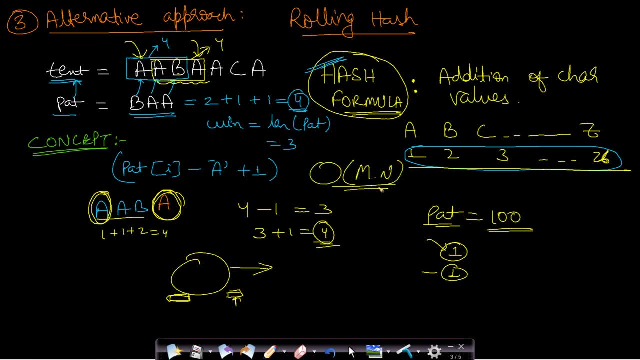 time. complexity of order of m into n. so this is better than your brute force approach, which was also mn, but the average time of this will be highly efficient than the brute force. but we can highly optimize this approach as well by taking a stronger hash formula so that the patterns do not 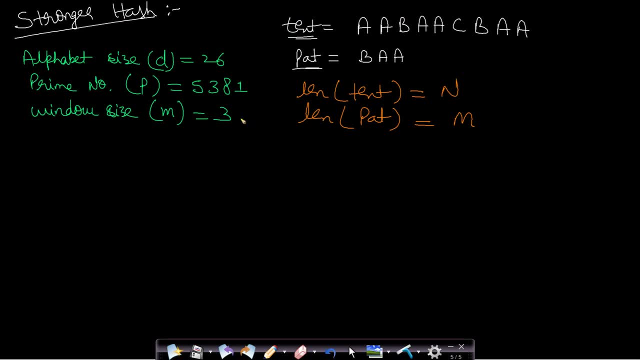 match easily, so let us look at how to form a stronger hash function. so we have taken the same pattern as well as the same hash, and length of text is n. length of pattern is m. now our alphabet size is 26. that is the number of times we have taken the same pattern as well as the same hash. and length of text is n. length of pattern is m. now our alphabet size is 26. that is the number. 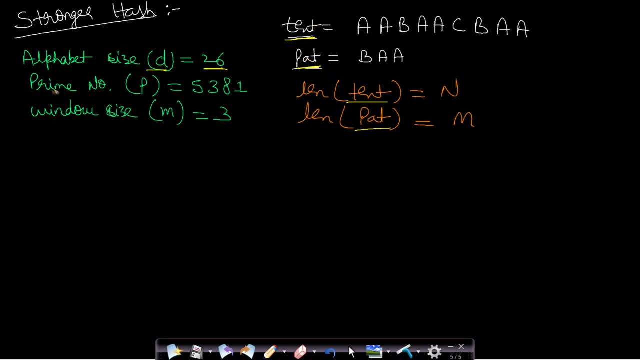 of unique characters which can be present in text or pattern. now the prime number taken is 5381. this is taken for taking the mod value so that the numbers do not overflow. you can take it as any prime number, but larger prime number means lower number of collisions. so this you should always. 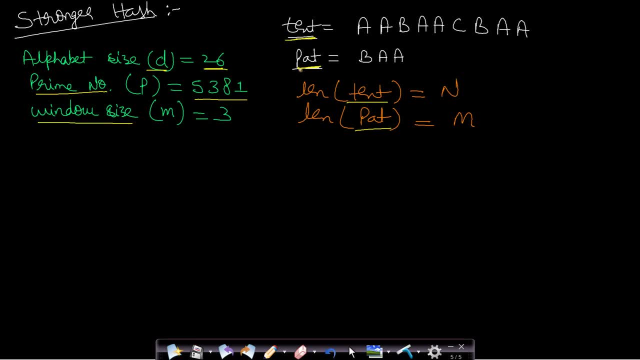 keep in mind. now, the window size here will be equals to the length of pattern. here the length of pattern is three, so window size will be three. okay, so these are the variables in order to form the stronger hash. so let's calculate the hash for this hash function. so let's calculate the hash for. 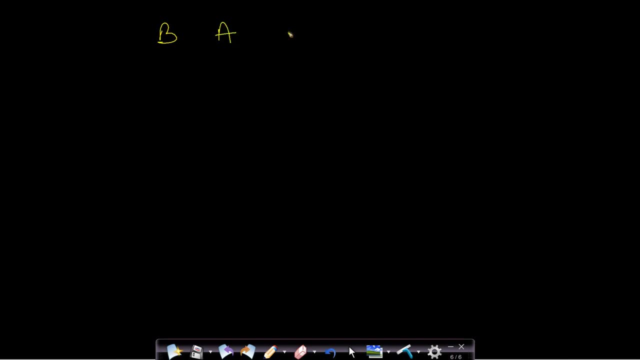 baa. now, if you want to calculate hash for baa, then what we will do is: for a, we will calculate the value, since we had already assumed that a will have value 1, b will have value 2 and so on. z will have value 26 and how it was coming. actually, if you are calculating for pattern at ith location, 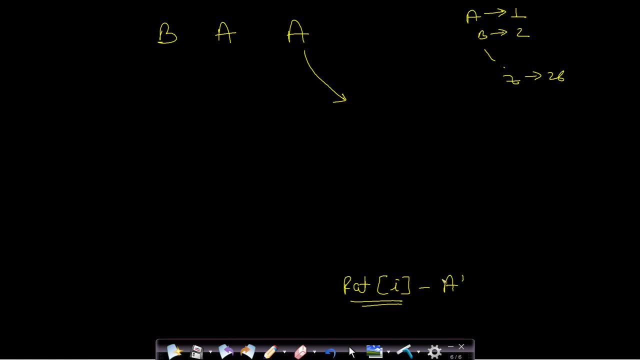 that is, this is the current character, then you will have to subtract a, which is the base character, and then add one to it. this will give you this integer value. now, once you have got this integer value, then we have taken here you can see we are. alphabet size is: 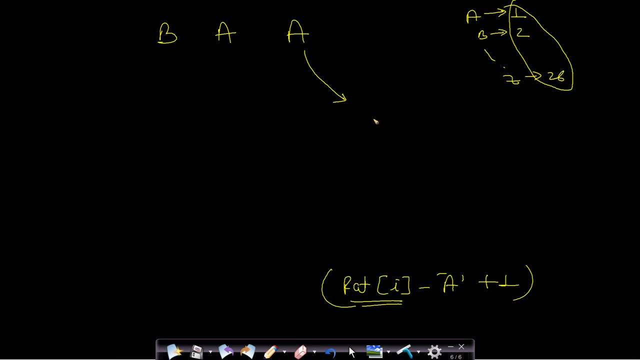 26. so we need to multiply it with the alphabet size and initially the power will be 0: power value. so here you will have to multiply 1 into 26 to the power 0, and then take a mod with p, which is our prime number. so in this second character we will have to multiply it by its value and power. 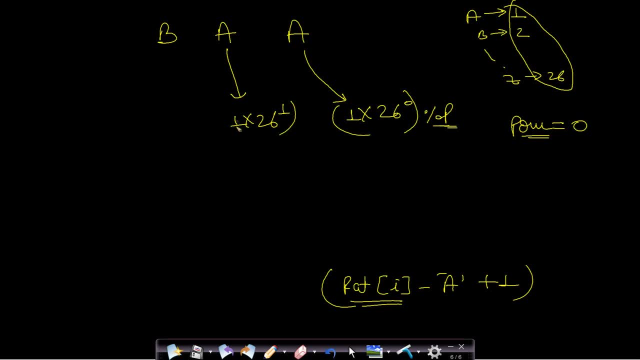 value, and this will be 26 to the power 1. and then you will have to again take a mod value with p and for this value as well, do the same. its value will come out to be 2. multiply it with 26 to the power 2.. so i hope you are getting the pattern now. and take mod with p now. how can we join all? 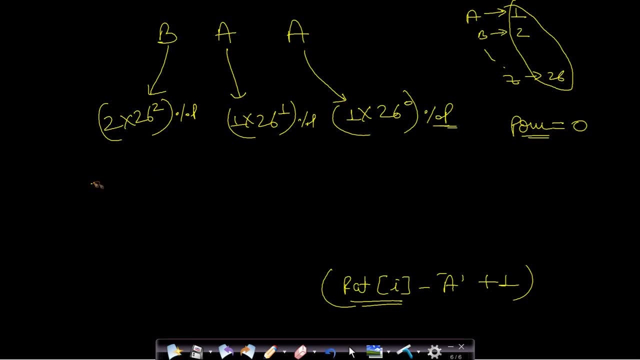 these values. basically, what will we do is we will have to take this 2 into 26 to the power 2 mod p. now this mod p is added with 1 into 26 to the power 1, and this is also taken as mod p. now this is added with 1 into 26 to the power 0. 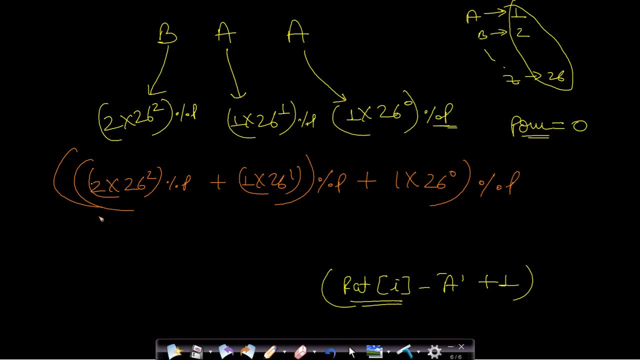 and entire value is taken with mod p. so this can be easily implemented by using a single for loop, and this code will be present in the code link which i will provide in the description below. so do check it out now, once you have calculated the hash of this baa, which will come out to be: 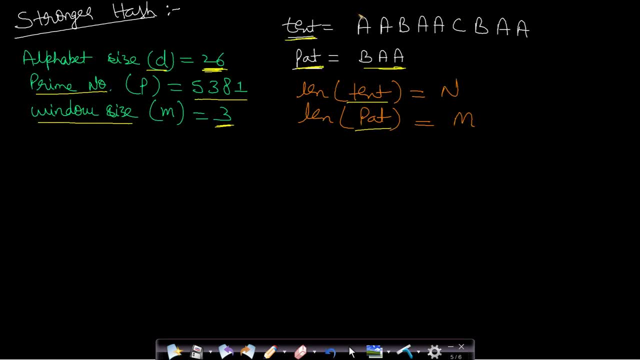 1379. i have calculated it already. you will take the first window, which is aab. now let us calculate the hash value of aab. what it will be, it's aab. so for a, your power values will be like 0, 1 and 2. 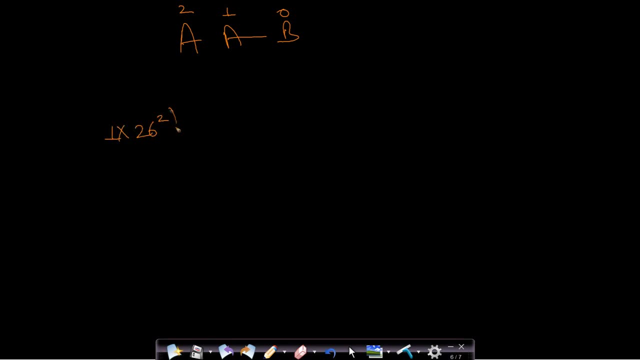 so for a value is 1 and you will take 26 to the power 2. this will be mod with p. now you will add 1 into 26 to the power 1, because value of this a is 1. so this will again be taken mod of p and for. 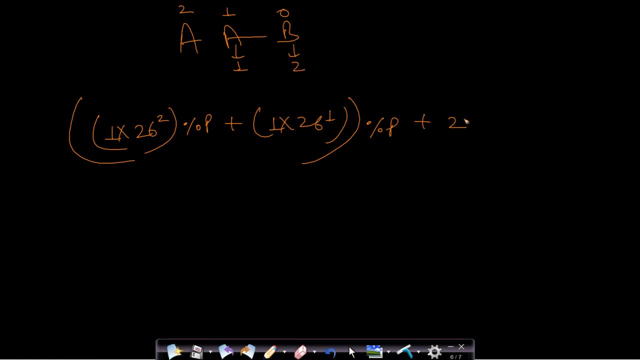 the third value, it will be 2.. will be added with 2 into 26 to the power 0, and the entire thing will be taken as mod of p. so once you calculate this entire value, then your value will come out to be 704. 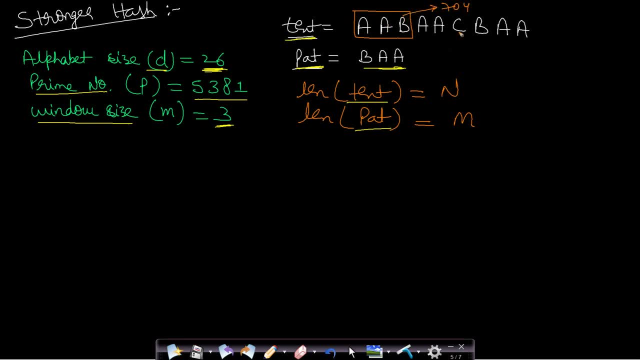 so here the hash value will be 704, and in this case the hash value was 1379. we will follow the same process as we did, only we have changed the hash function to make it a stronger hash. now, in our previous example you could see that for baa and aab. 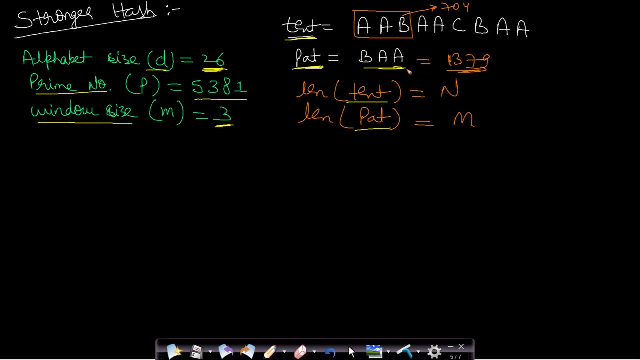 the hash values were matching, since we had taken only the additive hash, which was not at all a stronger hash in this case. you can see that they are far apart. they are not matching at all. so we don't need to match the characters. so you can see that. 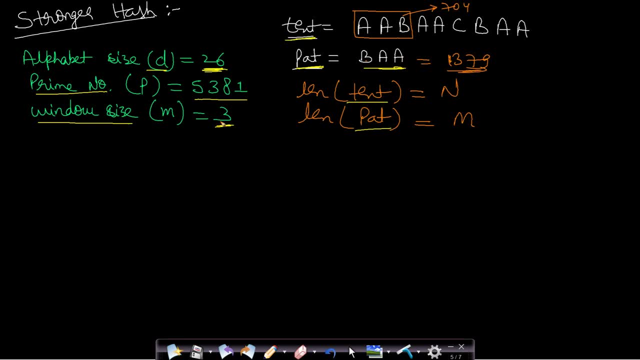 this will give a better result, so we will again repeat the same step. in this case, you can see that the hash values are not matching, so we will have to slide this window one value to the right. so how can we slide it? let's see for a, a, b, what was the value? this had power. 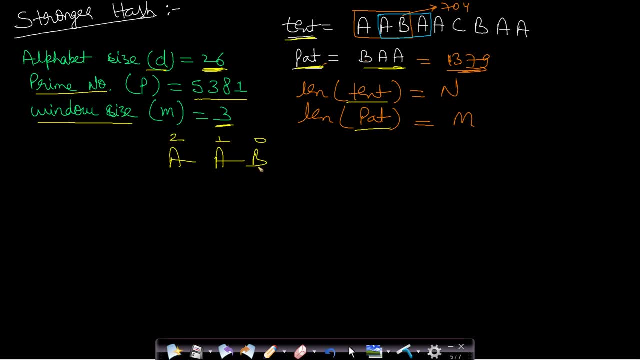 this had power 1 and this had power 2, as i had already shown. so once you leave this character and once you add a new character, then first of all we need to remove this character. so what was the value for this character? it was 1 into 26 to the power 2, and this was modded with p. so you need 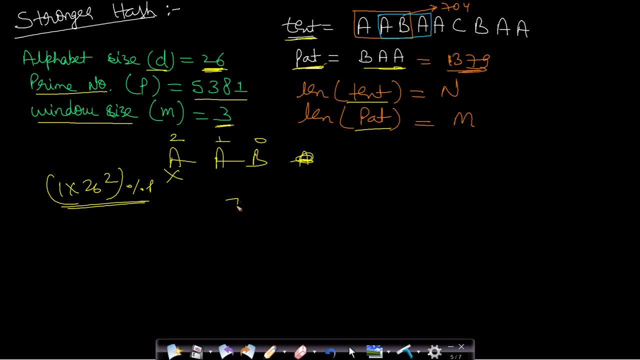 to subtract this value from this entire value. so it will be 704 minus 26 to the power 2. 1 into 26 to the power 2. this will be subtracted and the value which will come is 28. this is the value for. 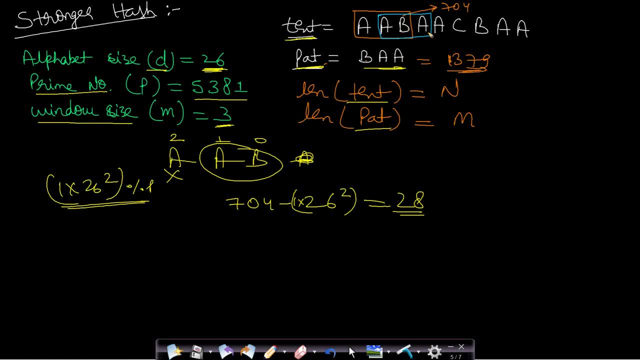 only a- b. now what you need to do is you need to add this a on the right hand side. for this you need to left shift this a- b. so for your clearance in the base 10 number system, if you have a number, let's say 28, and if you want to like left shift by one bit, then you need to multiply it with the. 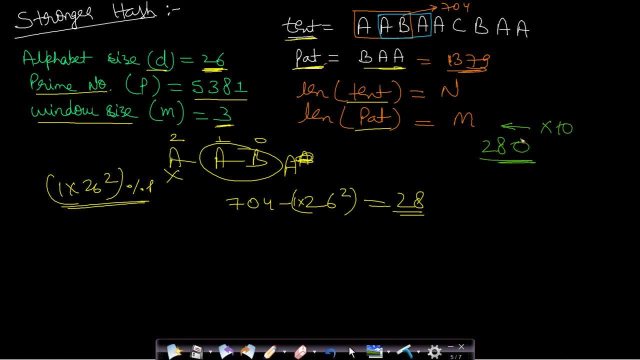 base value, which is 10, and then it will become 280. so it has shifted by one value to the left hand side. this is a base 26 number. okay, i have already assumed that the alphabet size is 26. so in order to shift it to the left hand side by one value, then we will have to multiply it with the base. 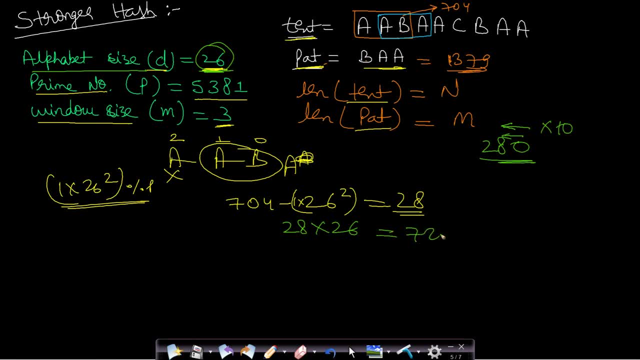 value, it will be 26, so this will come out to be 728, i guess, and then, once it has been shifted, then we can add this rightmost value, which is a, so a's value is 1- into 26, to the power 0, which. 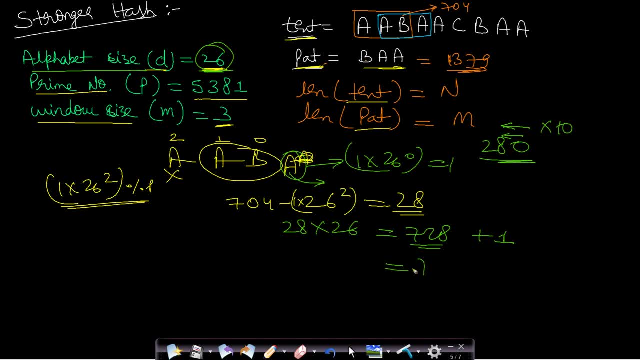 is equals to 1, so we will add just 1 to it. it will be equals to 729. so this is the new hash value of this window, which is 729. now again, these values are not matching, so we will again slide it to the right hand side. so in this way you can see that this. 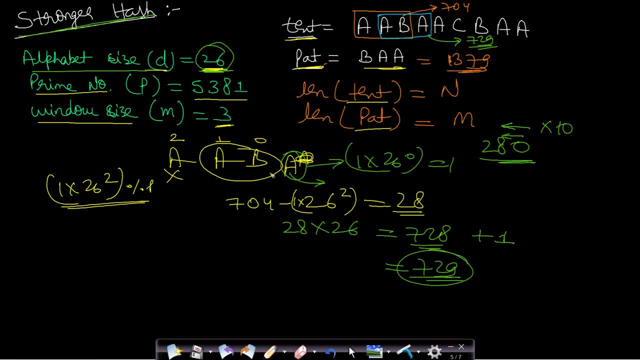 is a lot stronger hash as compared to our additive hash. in the worst case, the time complexity will be same, which is order of mn, but the average time will be much less, much, much lower than the brute force as well as the efficient approach in our this additive hash. so this is all about the rolling 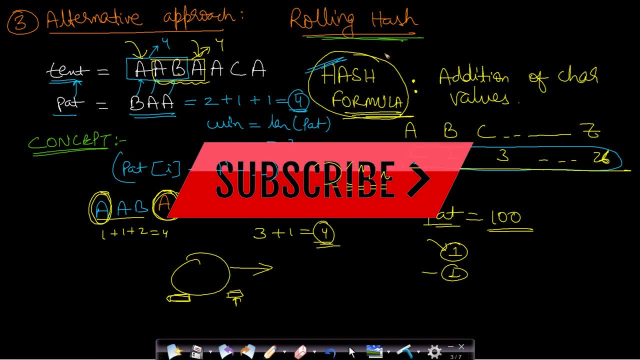 hash and the ribbon carp algorithm. so this is the new hash value of this window, which is 729. now again, this is the new hash value of this window, which is 729. so this is the new hash value of this window, as well as the pattern searching using it. so i hope i was able to make you understand the concept of.